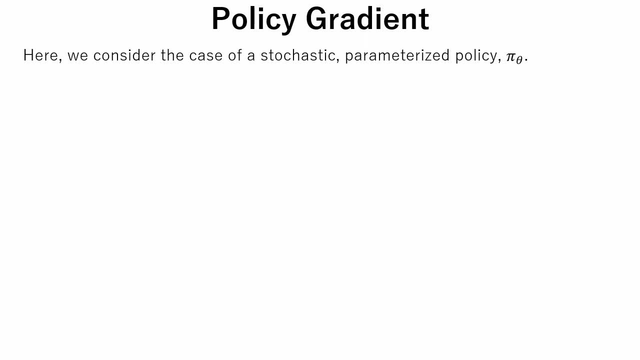 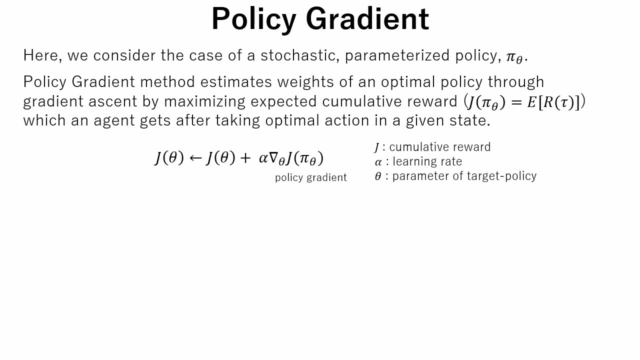 Here we consider the case of a stochastic parameterized policy. pi-theta Policy gradient method estimates weights of an optimal policy through gradient ascent, by maximizing expected cumulative reward which an agent gets after taking optimal action in a given state. To actually use this algorithm we need an expression for the 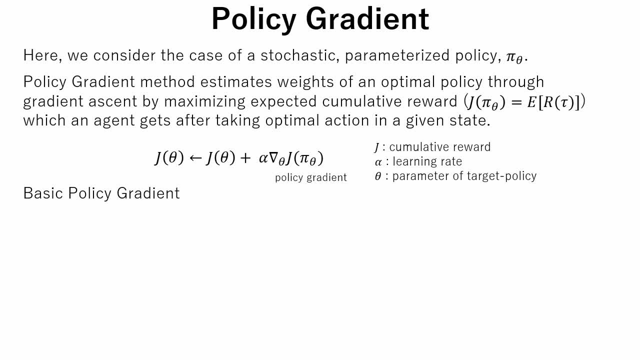 policy gradient, which we can numerically compute. After several expression transformations, we can get this formula. This is basic policy gradient. In this form, policy gradient can be estimated by letting the agent act in the environment using the policy and collecting a set of trajectories. 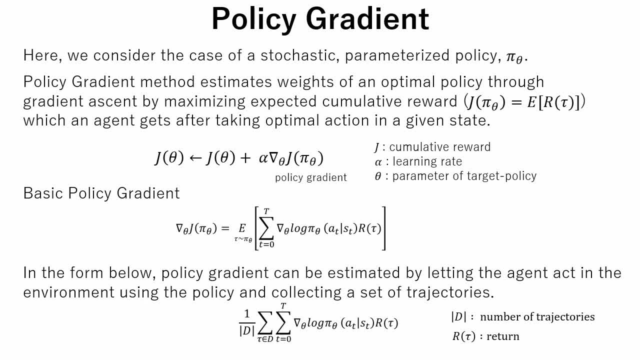 This is the simplest version of the computable expression. In the case of deterministic policy gradient method, we can use the formula to calculate a set of trajectories. This is the simplest version of the computable expression. As is the case with deterministic policy gradient method, 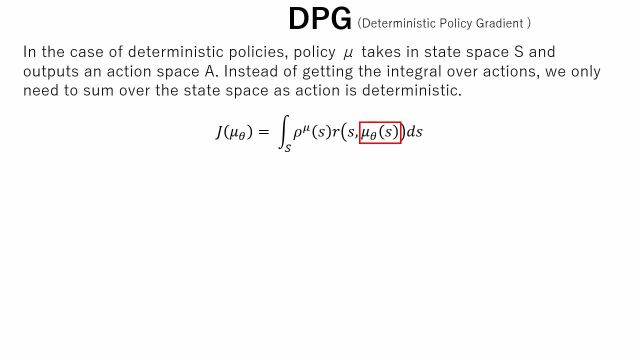 the policy takes in the state space S and outputs in action space A. Instead of getting the integral over actions, we only need to sum over the state space, as action is deterministic. This is an expanded form of the deterministic policy gradient. The proof for this deterministic policy gradient is similar in culture to 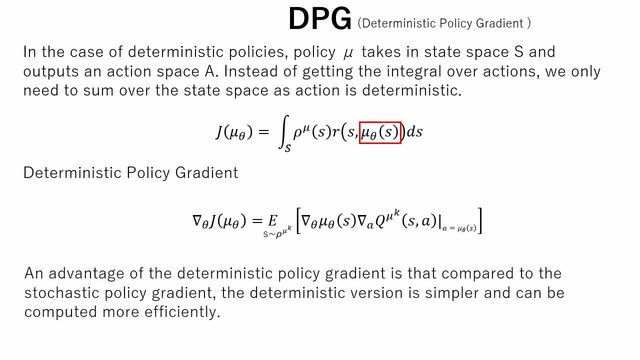 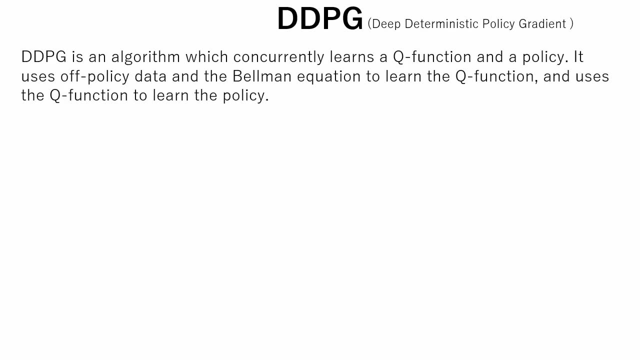 the proof for the policy gradient theorem. An advantage of the deterministic policy gradient is that itき is down to these expressions- is that, compared to the stochastic policy gradient, the deterministic version is simpler and can be computed more efficiently. DDPG is an algorithm which, concurrently, 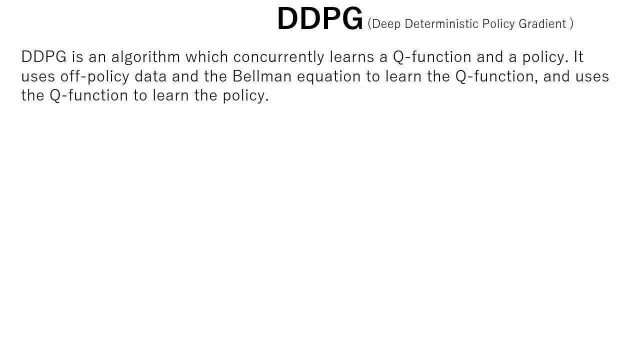 learns a Q function and a policy. It uses off-policy data and the Bellman equation to learn the Q function and uses the Q function to learn the policy. Now I will explain some facts behind the two parts of DDPG: Learning a Q function. 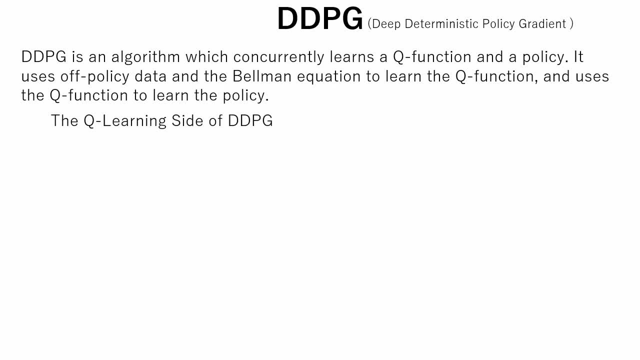 and learning a policy. Let's begin from the Q learning side of DDPG. In DDPG we are using mean squared Bellman error function, which tells us roughly how closely Q phi comes to satisfying the Bellman equation. Here small d indicates whether 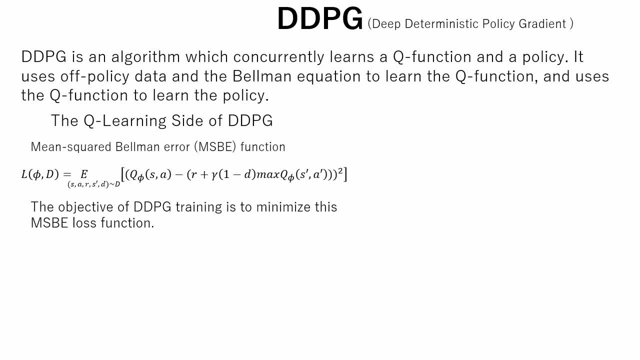 the next state is terminal. So the objective of DDPG training is to minimize this mean squared Bellman error loss function. There are several methods used to successfully train the network. The first is replay buffer. This is the set of previous experiences. In order for the algorithm to have stable behavior, the replay 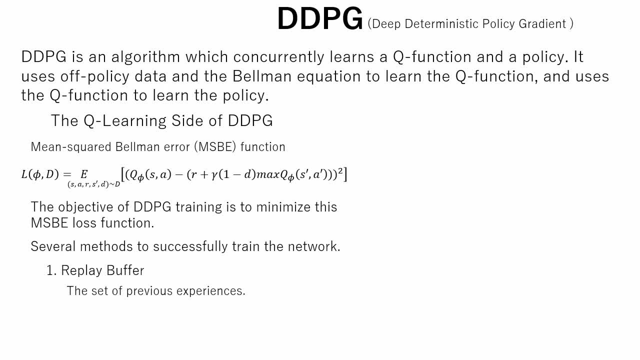 buffer should be large enough to contain a wide range of experiences. But if we use use too much experience, you may slow down the learning. The second is target network. By using target network we can stabilize the learning In DDPG style algorithms. 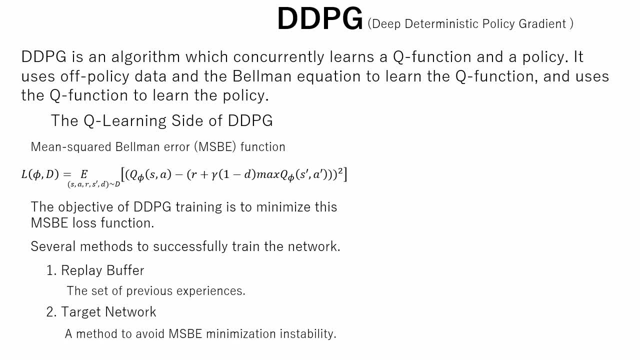 the target network is updated once per main network update by Polyac averaging. Now about the policy learning side of DDPG. Policy learning in DDPG is fairly simple. The objective is to learn a deterministic policy by theta which gives the action that maximizes Q phi. 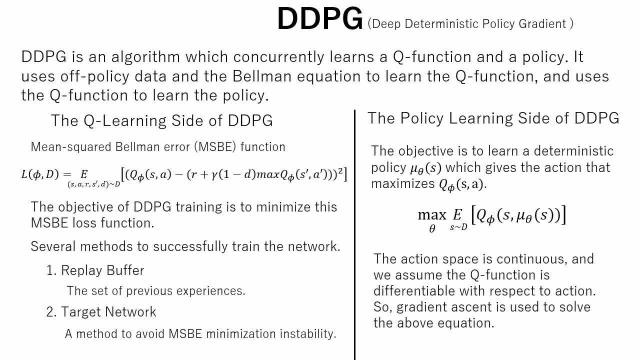 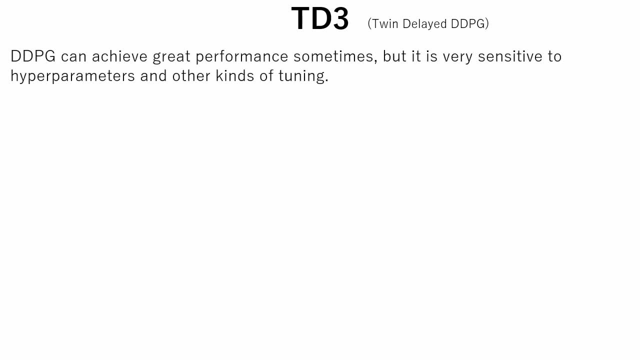 The action space is continuous and we assume the Q function is differentiable with respect to action. So gradient ascent is used to solve the above equation. Finally, we get to TD3.. DDPG can achieve great performance sometimes, but it is very sensitive. 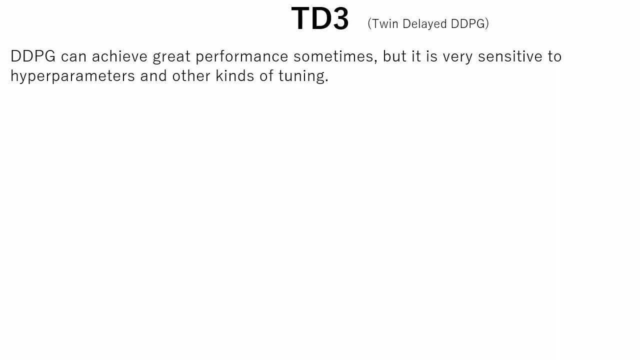 TD3 is very sensitive to hyperparameters and other kinds of tuning. Often learned Q function begins to dramatically overestimate Q values, which then leads to the policy breaking because it exploits the errors in the Q function. TD3 overcomes this issue by introducing three critical tricks. 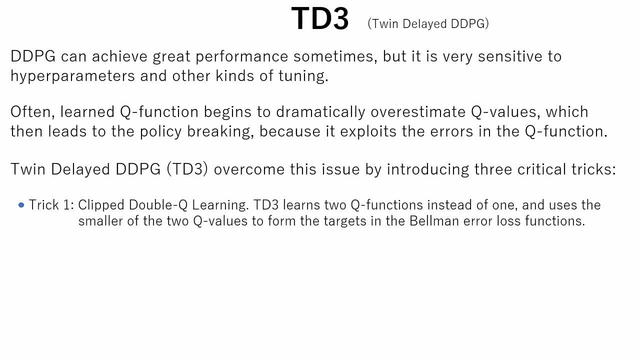 The first is clipped double Q learning. TD3 learns two Q functions instead of one and uses the smaller, which is the first of the two Q values, to form the targets in the Bellman error loss functions. The second is delayed policy updates. 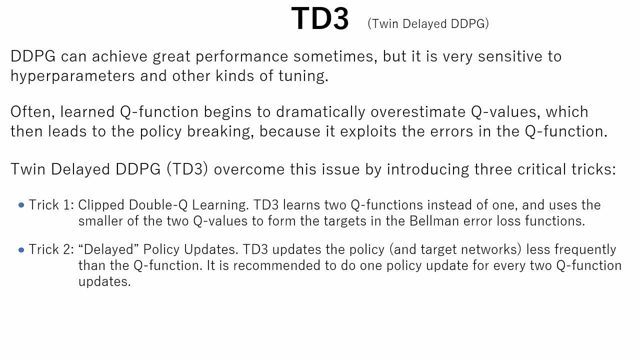 TD3 updates the policy and target networks less frequently than the Q function. It is recommended to do one policy update for every two Q function updates. The third is target policy smoothing. TD3 adds noise to the target action to make it harder for the policy to be moved. 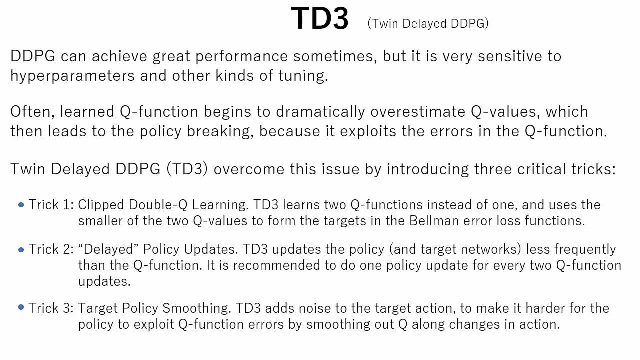 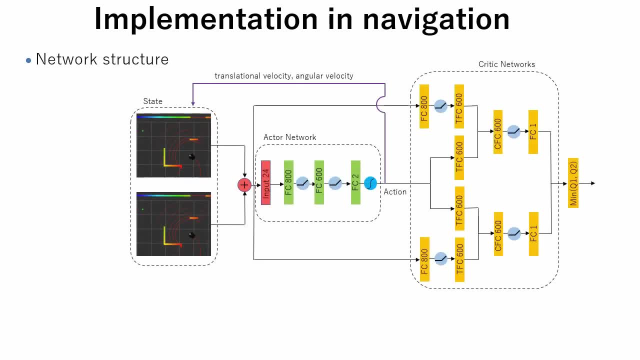 The fourth is the ability to exploit Q function errors by smoothing out Q-along changes in action. Here is a structure of a network we used in this simulation. Robot states consist of distance between robot and goal angle, theta between robot heading direction and goal direction. 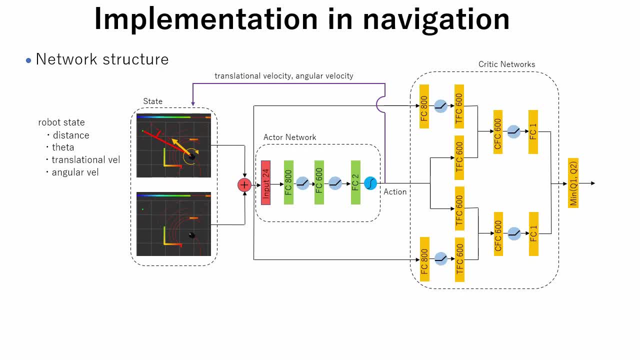 translational velocity and angular velocity of the robot. It also contains distances to obstacles, each 9 degrees and 180 degree radius. очки добавис are now running in range in front of the robot, As has been described in the previous slide. 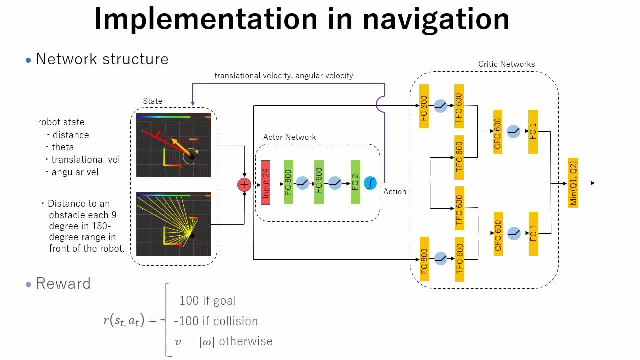 Clipped double Q learning trick is used in this network. so there are two identical networks. in one critic network The policy gets reward of 100 if the robot reaches the goal and gets minus 100 reward if collision happens, Also each time step. 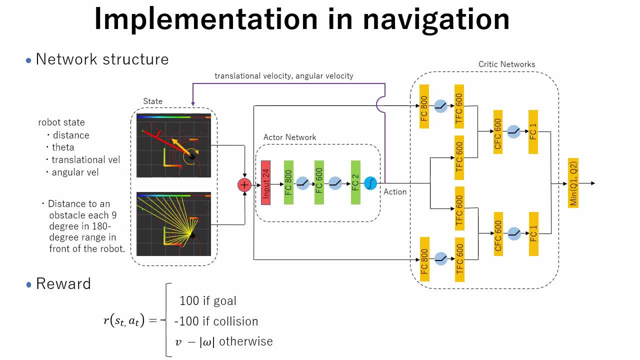 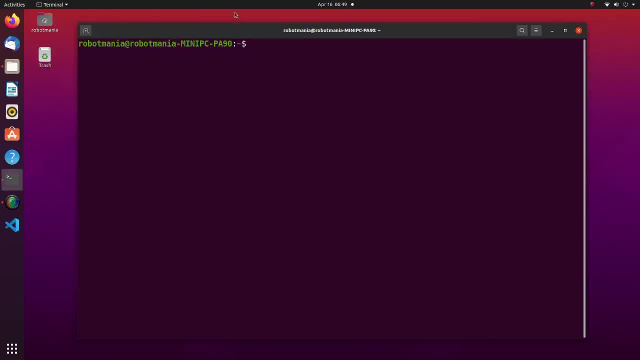 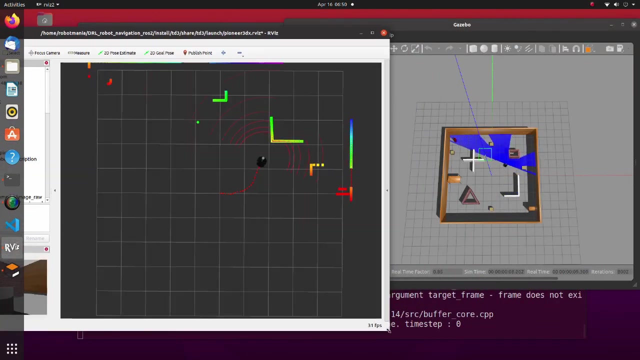 the robot gets reward. This reward is applied to make the robot move forward as much as possible. Now let's execute the simulation. Firstly, we have to train our network. To do this, launch the training simulation launchpy script To observe how training goes. TensorBoard is helpful. 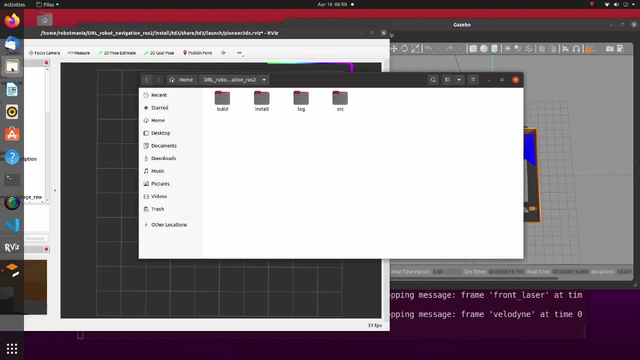 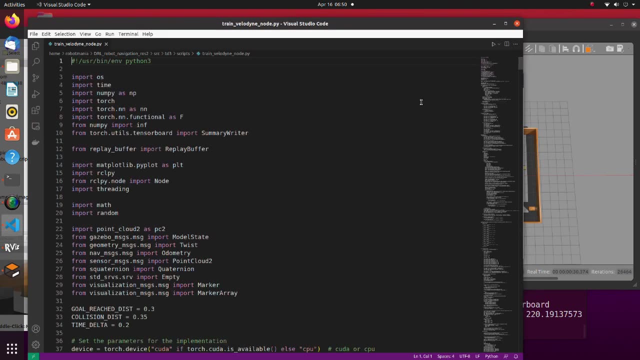 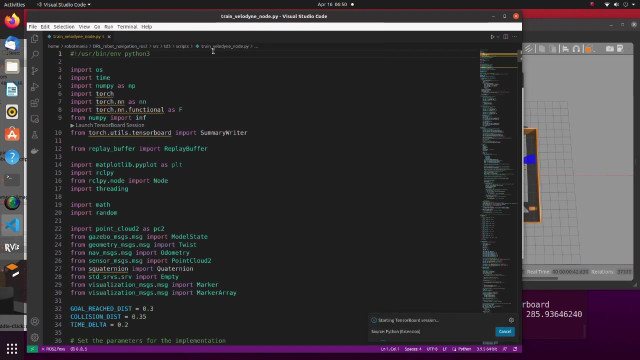 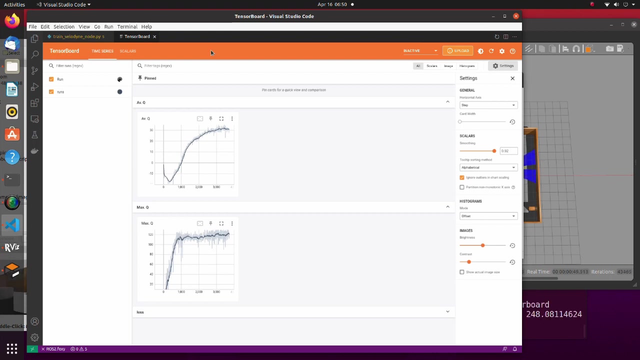 Open train Velodyne nodepy script using Visual Studio Code. Launch the TensorBoard board. Select current directory. Note that the graph here is describing the state after the training is complete. Here we can see that it takes about 3700 steps for Q average value to converge.